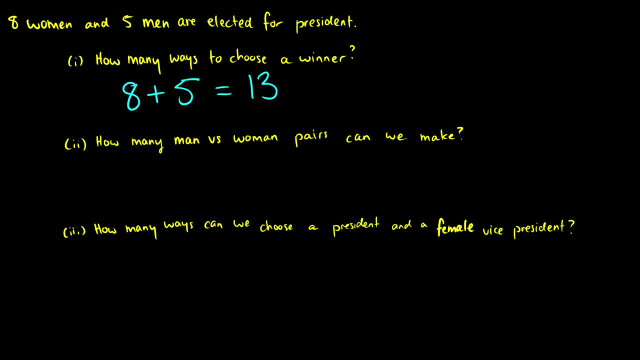 them up into cases of men and women. so either a woman can win or a man can win. therefore, 8 plus 5 is 13.. Okay, so how many man versus woman pairs can we make? So let's pretend it's going to be one. 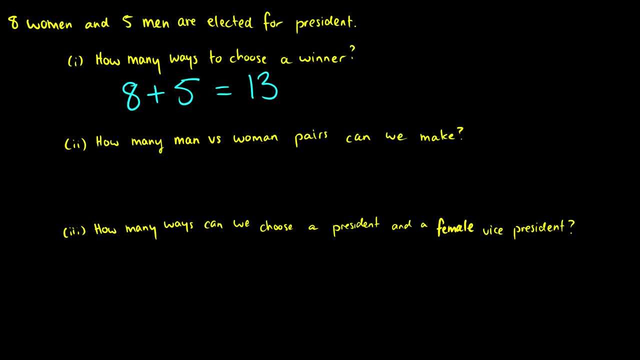 woman up against one man. So for the men, there's five choices for the man to be in our pair, and then there's going to be eight choices for the woman. So we're going to have 40 pairs. Now, this uses the rule of product. 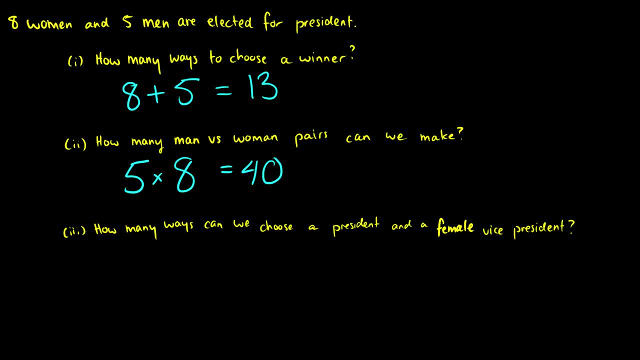 because we're choosing a man out of our pool of five and then we're choosing a woman out of our pool of five and we're pairing them up. So each man is going to be paired with each woman, or has the possibility to be. So we choose a man and then we choose a woman. 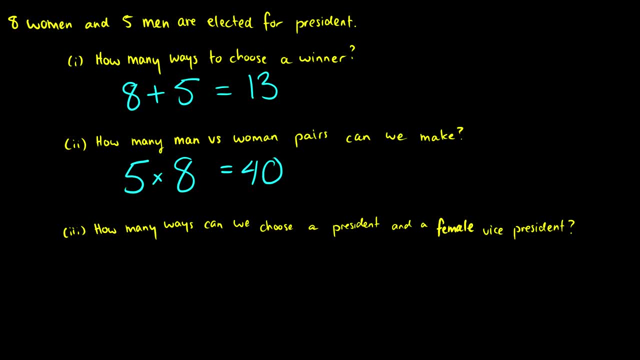 So it's five times eight is 40 possible pairs. Okay, how many ways can we choose a president and a female vice president? So first we're choosing a president and then we're choosing the vice president, but that vice president has to be female. Okay, so let's take a look here. 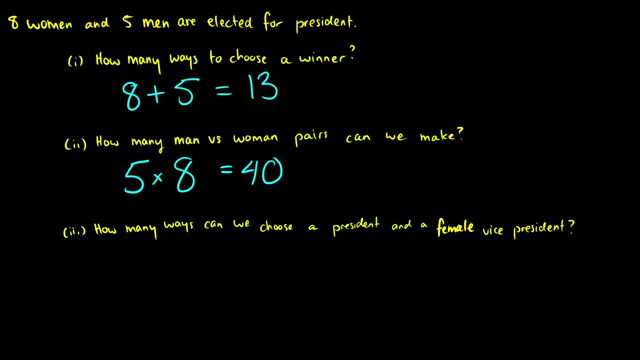 How many ways can we choose a president? Well, let's think, here there's 13 candidates for a president, So we choose one of those 13 candidates and then we need to choose a vice president. Well, here is the problem. If our first president is female, then our second choice for vice president is: 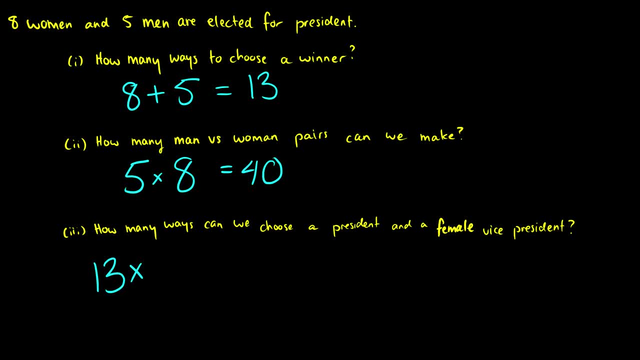 going to have one less woman in the pool, But if our president is male, then we have all eight women to choose from. So maybe we shouldn't say it's 13 times something. Maybe we should break this up and say: look, we have a male president or a female president. So our first scenario here: 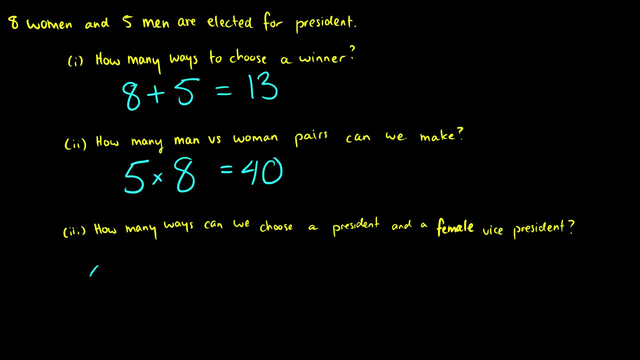 we have a male president. Let's do that. We choose a president from the men, That's five- And then we choose a female vice president. So now we have eight possible choices. So this is our male female vice president, And then we're going to have a female female pair. So we have eight choices for 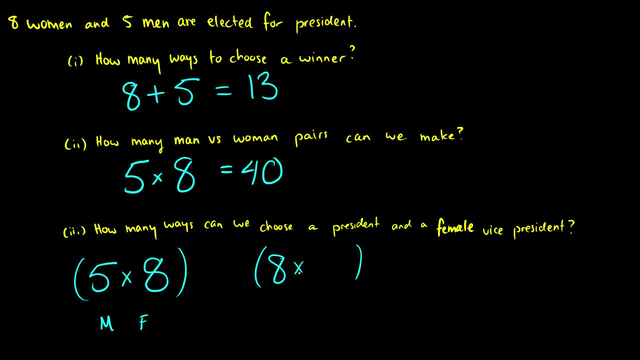 a woman as president, And then we have seven choices for the remaining woman as president. So this is the F and F combo And we're saying: look, it can be male and female, or female, female. So we use the rule of sum to add these two conditions together. So our end result is going to 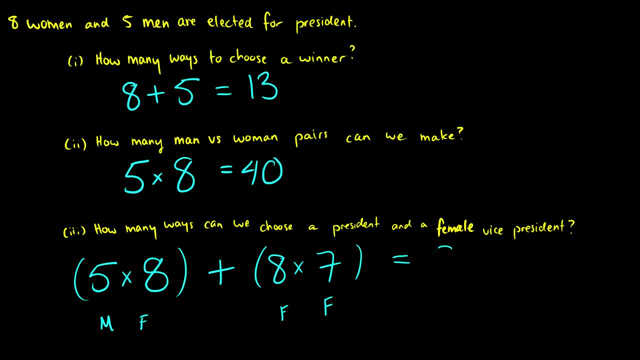 be 40 plus 56. Which is 96 possible pairs. So this is a nice example of how you can take a very simple problem and make it a little bit more difficult. If we said: choose a president and a vice president, that'd be easy because we 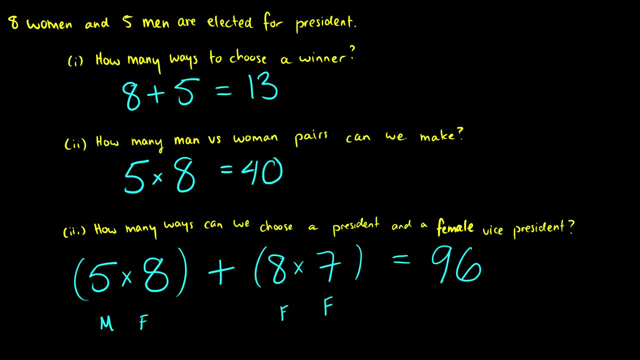 have 13 possible choices for the first and 12 for the vice president. But this gets a little bit more difficult because we're putting this constraint on the vice president And one of those situations we might be using up in the first If we just start with 13, saying okay, look, it can be any. 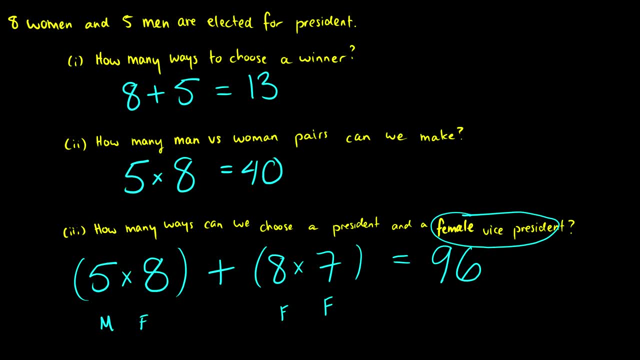 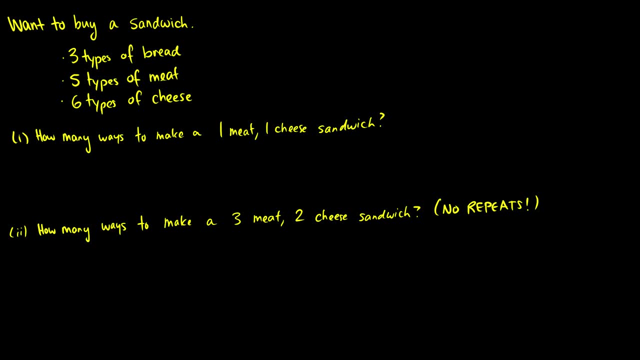 of these 13, and then you break the vice president up into cases not too easy. There's the first question. Second question: We want to buy a sandwich And this store has three types of bread, five types of meat and six types of cheese. So how many ways can we make a one meat, one cheese? sandwich. Well, first we choose our type of bread. It says two, However that stands for three, so that is going to cost a lot of money because we're using so much different sources for the first, and then how manyhmares we make up, And then five or six types of meat. I hope we don't get a lot of demand for a tablespoons sometimes. 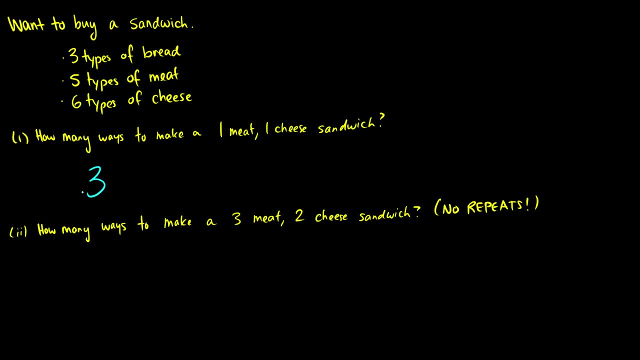 Let's just start right here, So wait a second. So if we choose our types of bread, I'm just going to start with our type of bread- So there's three types. Then we want to choose our meat, So there's five types we can choose from. Then we want to choose our cheese: There's six types. to 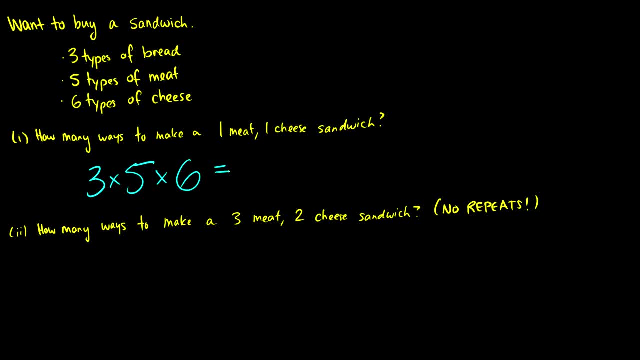 choose from. So we have three bread, five meat and six cheese to choose from, which means we have a total of 90 combinations. This is just like the ice cream problem in the previous lecture, video Two: How many ways can we make a three-meat, two-cheese? 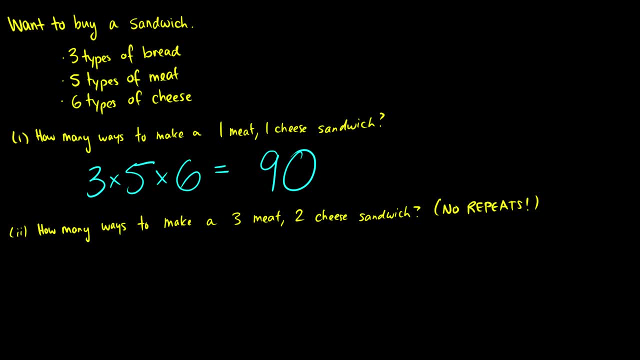 sandwich and we don't want any repeats. Okay, so first we choose our type of bread And now we want three meats. So we have five choices for our first meat, We have four choices for the second meat And we have three choices for the third meat because we want three.